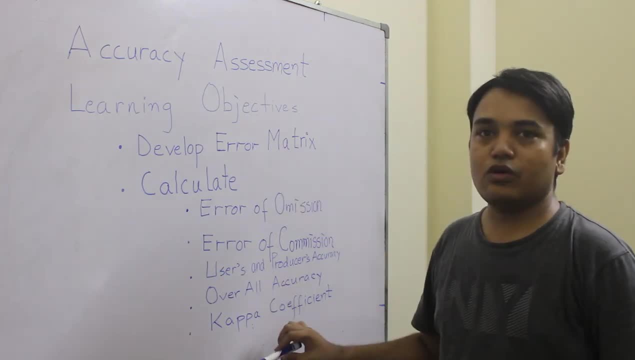 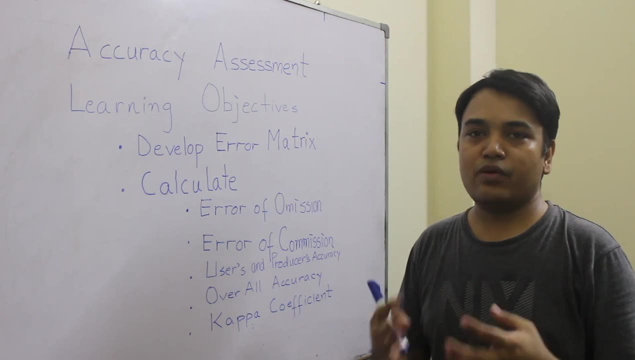 So in this video we will go through all these steps. So first of all, what we will do is understand an error matrix. We will do all this mode And then we will sit on your computer and calculate all the statistics, which includes commission error, user accuracy, overall accuracy and kappa coefficient. 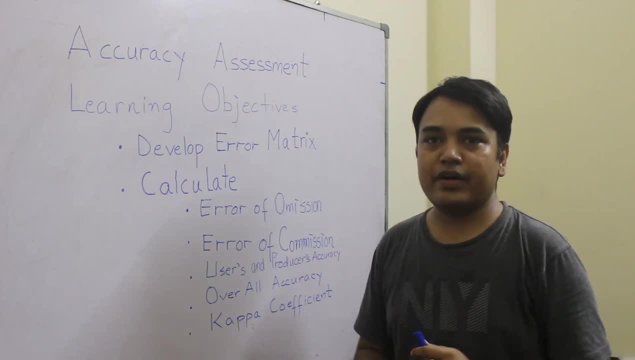 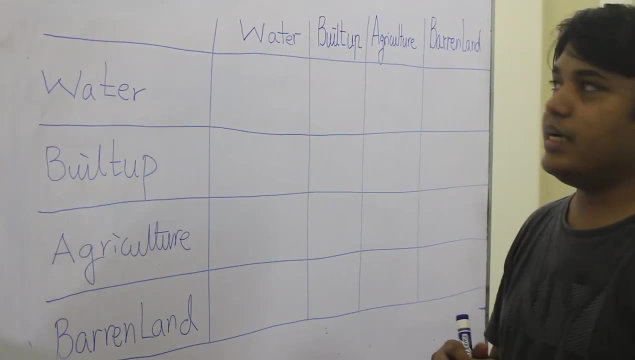 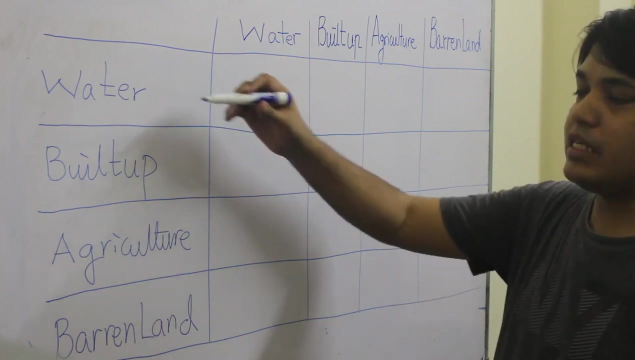 Let's first see what is error matrix. So what we will do is basically understand the error matrix. So now let's understand error matrix. And in error matrix, what we have is basically the classes which is classified in the classified image: Water buildup, agriculture and management. 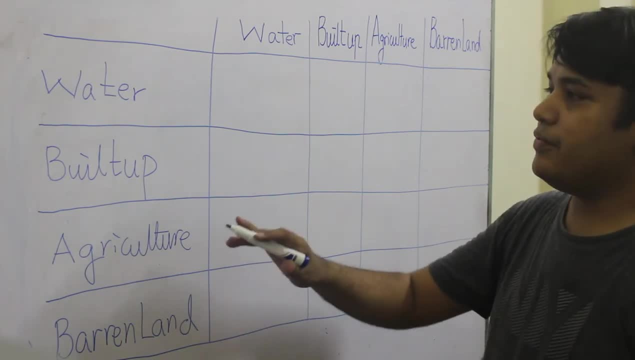 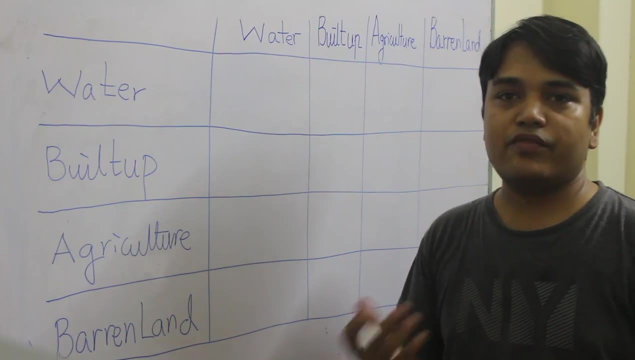 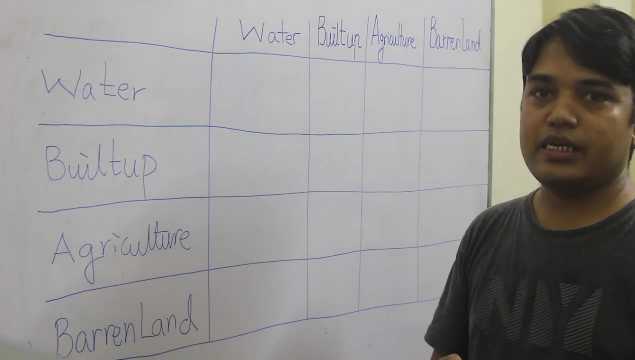 So it's basically a matrix between the classified pixels with the reference pixels, And the reference pixels are those pixels which you got the data from the ground. You go to the site, select one specific location, get the data and see what is the error matrix. 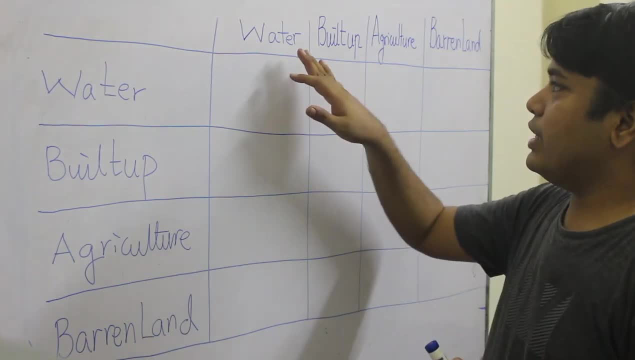 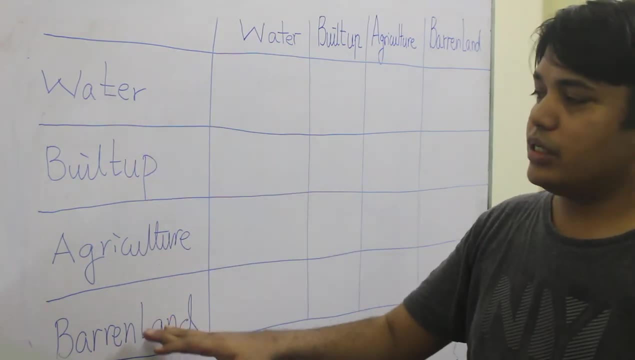 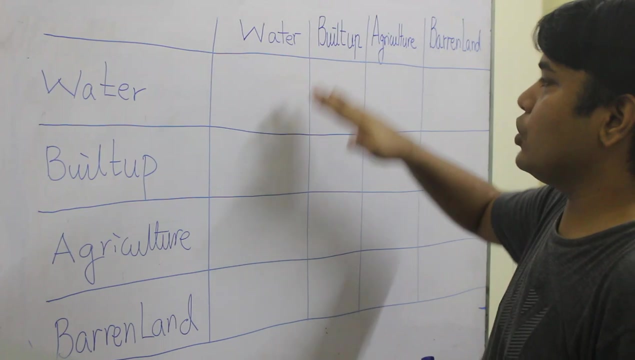 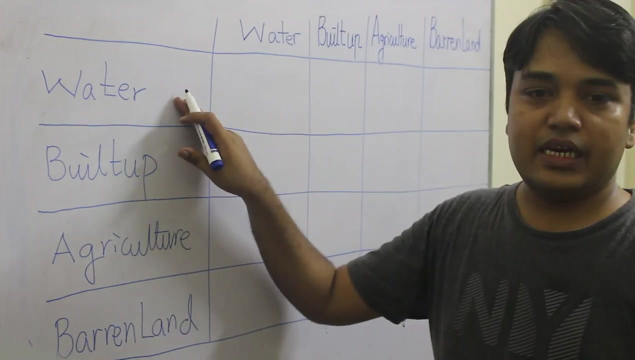 And then you can see what it is in respect to water buildup, agriculture or management. So what rows shows here are basically the classified pixels, And what column shows are the reference size pixels. So now let's suppose for the water we had a total of 43 pixels. 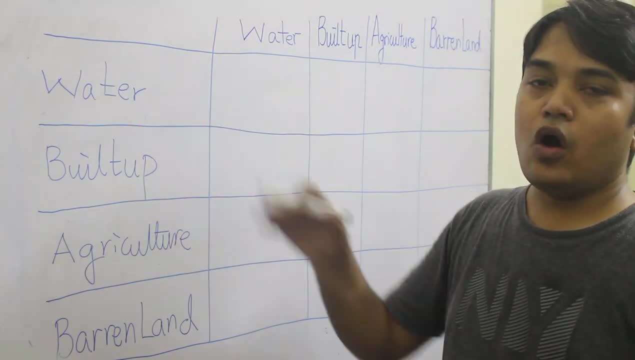 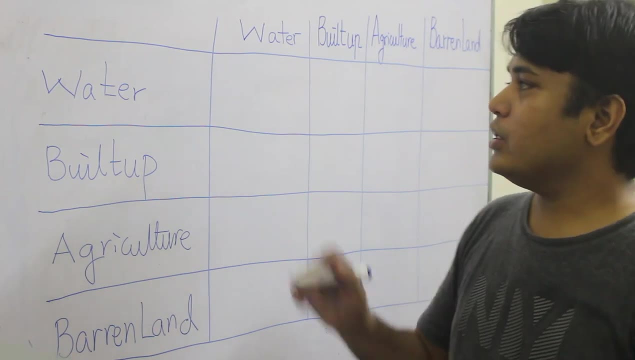 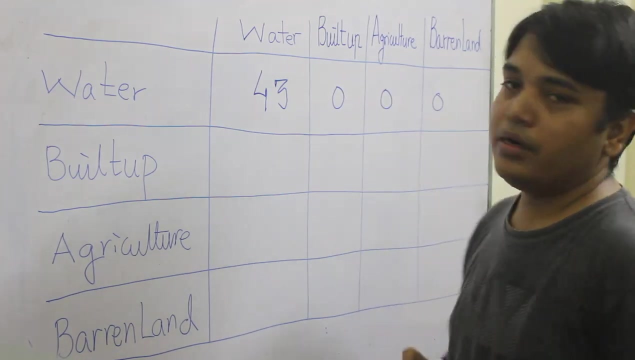 And out of 43,. all of the 43 were correct And when we went to the field we found out that those are water. So we will write 43 here and 0 at all on the columns. Then, coming to the buildup, 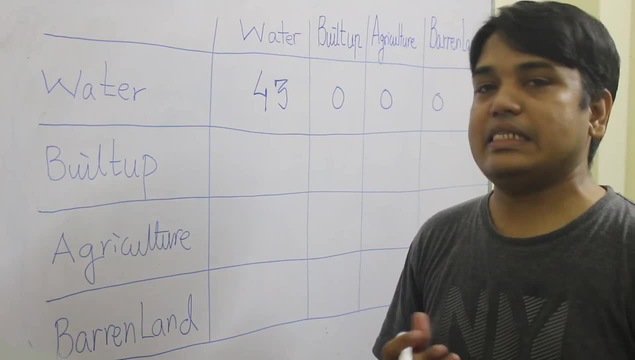 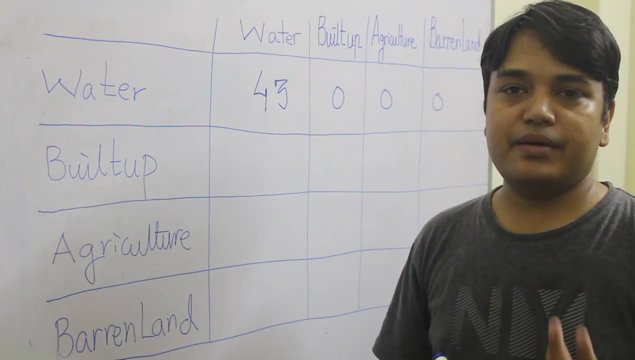 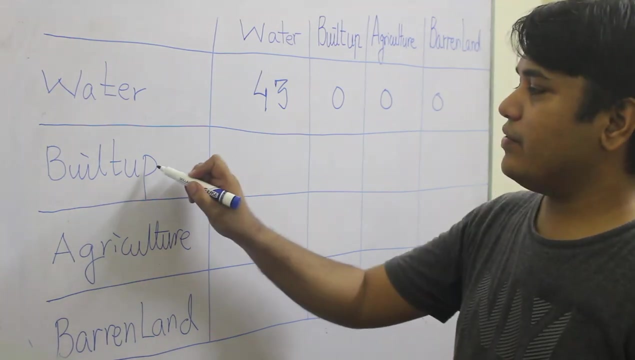 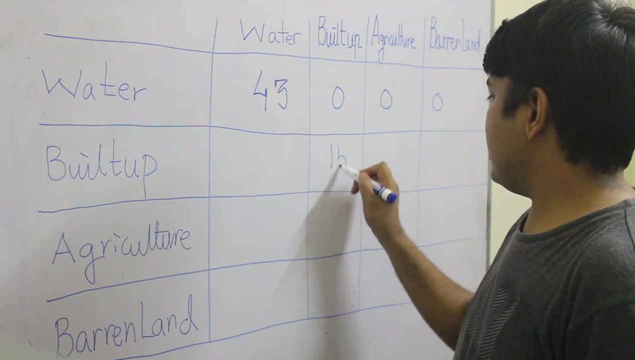 So at the buildup we have a total of 16 pixels, 16 classified pixels. So by reclassifying the image we found out that in total 16 were classified But 15 were on the ground buildup. But one was a barrier. 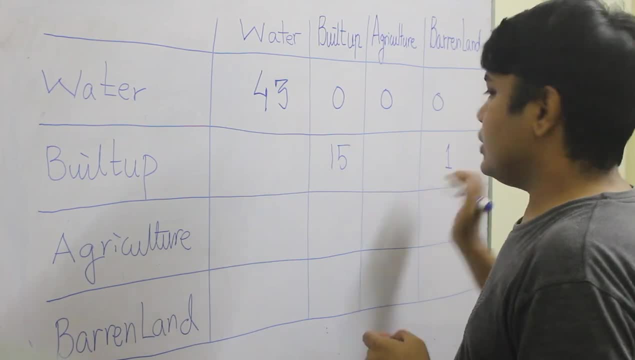 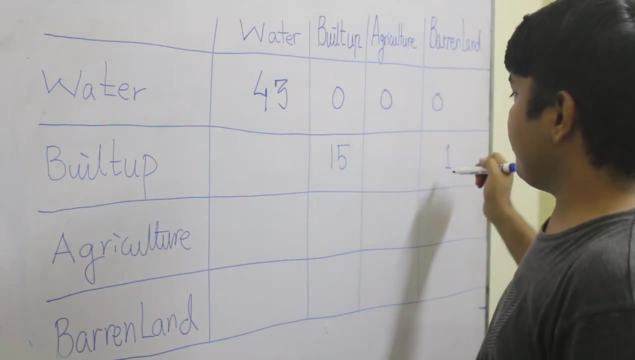 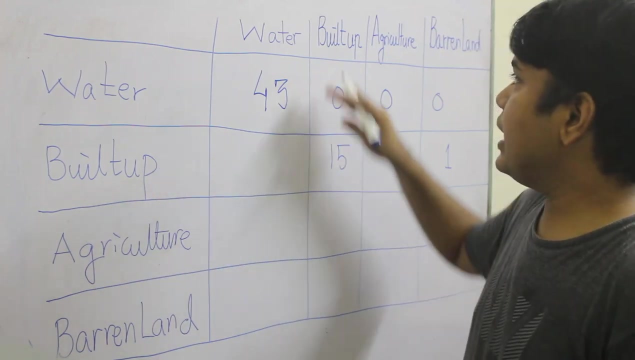 So we will put it here as well. So in total we classified. We classified 16 images, But on ground we had 15 buildup and 1 barrier. So just to understand like the rows will show you the classified information And the columns will show you the reference of the ground coding information. 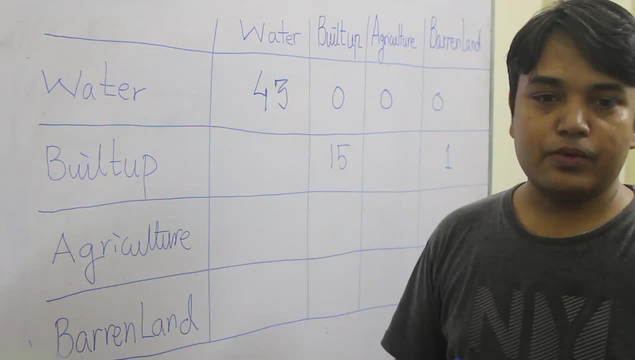 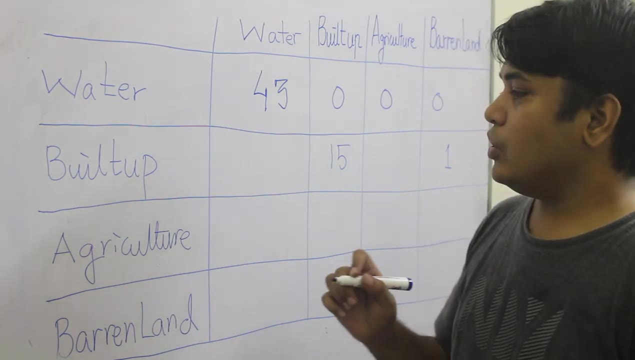 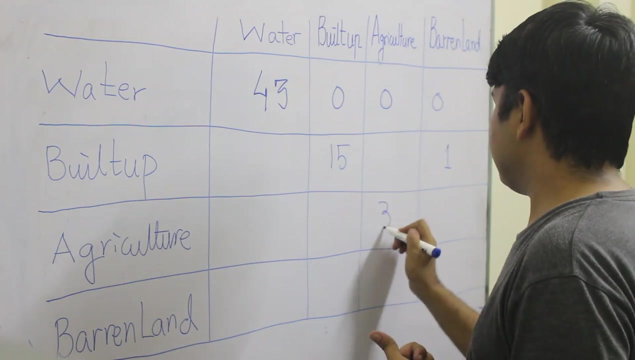 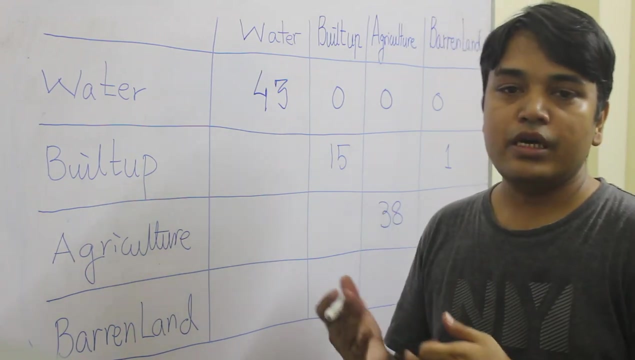 And then, coming to agriculture, Suppose we had agriculture. In total there were like 43 pixels. So out of 43 pixels, 38 were in agriculture, On the ground. So the 38 classified pixels were same as on the ground, But 5 were not in agriculture. 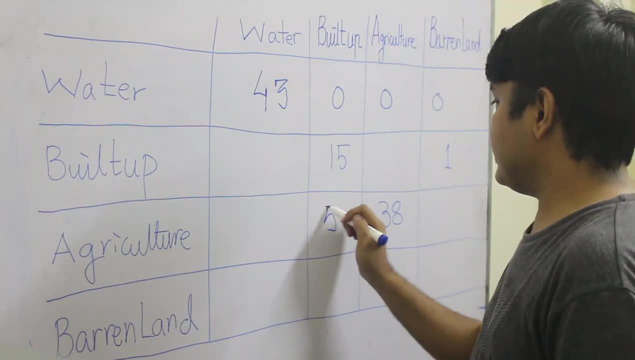 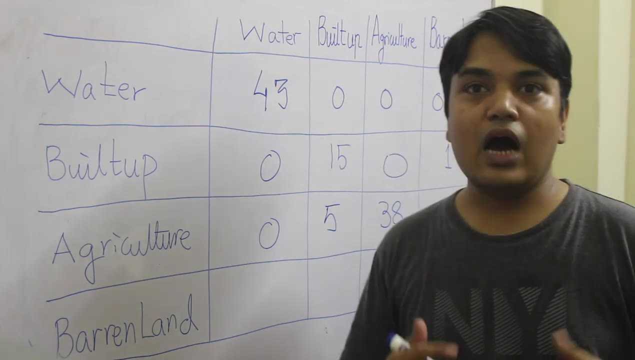 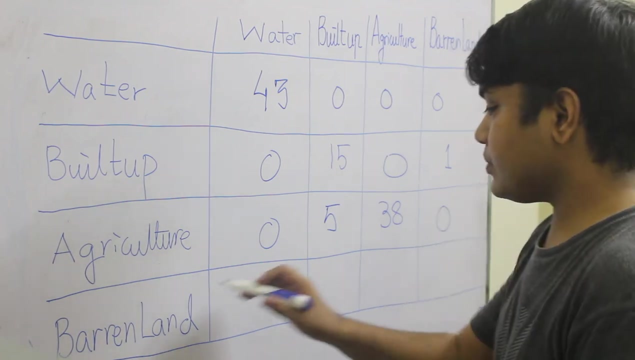 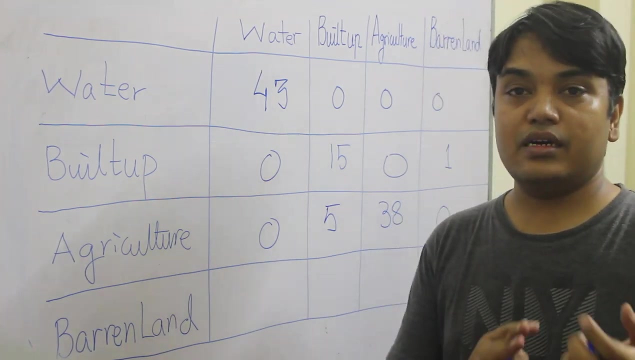 They were buildup, So we will put 5 here And 0 for the less colors. And now coming to the barrier, So in total barrier there were 40 pixels. So you see there were 40 pixels in total And out of 40, 39 were correctly classified. 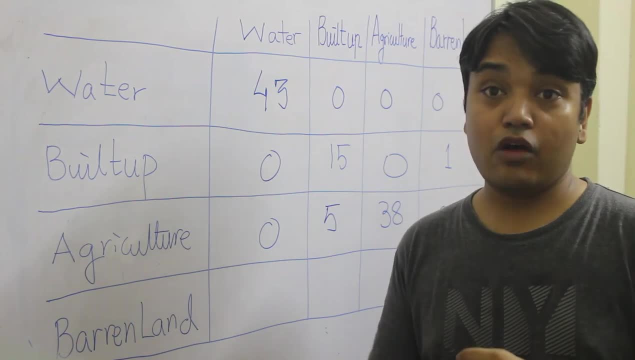 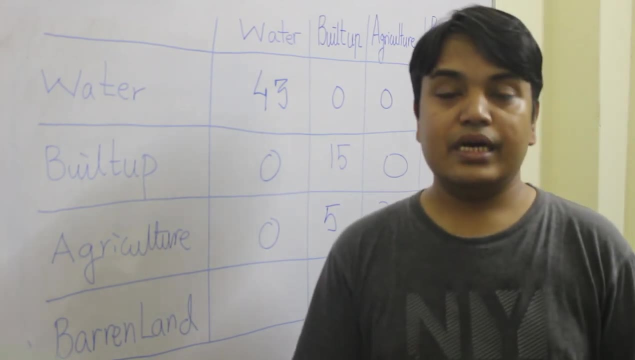 For example, classified pixel was also a barrier And on the ground it was also a barrier. So we will write 39 here And 1 was basically a buildup on the ground. So it was classified as a barrier, But it was buildup on the ground. 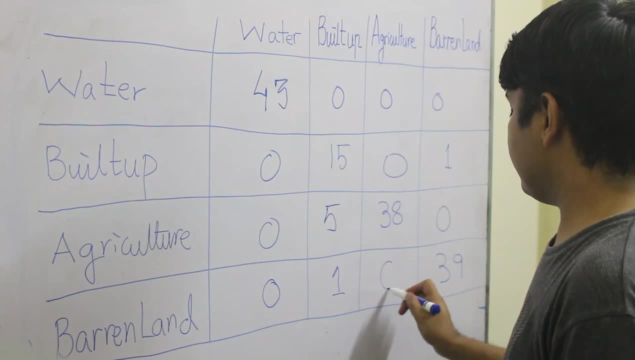 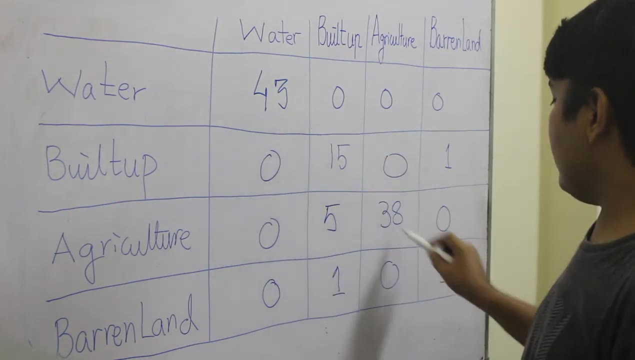 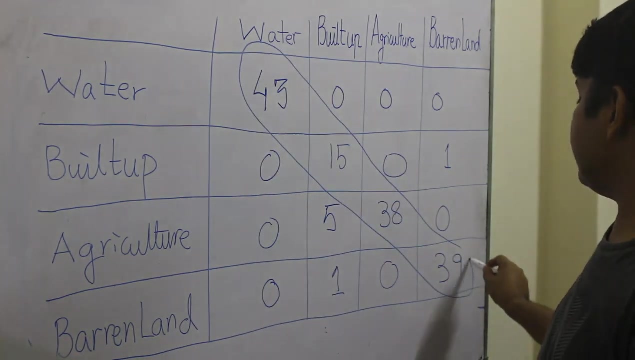 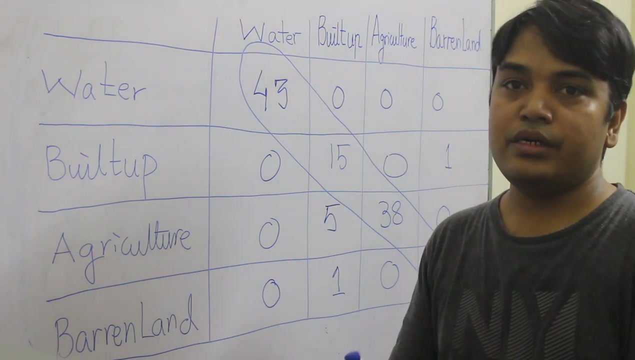 So we will put 1 here. So you will see one thing in this matrix. So all the diagonals are basically those pixels Which are classified correctly, And these are same as it is on the ground, Which is what we get from using any classification scheme. 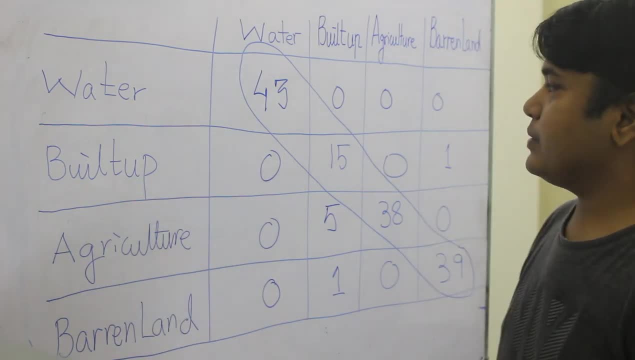 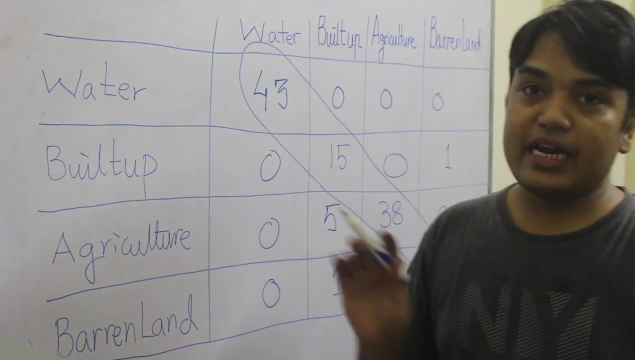 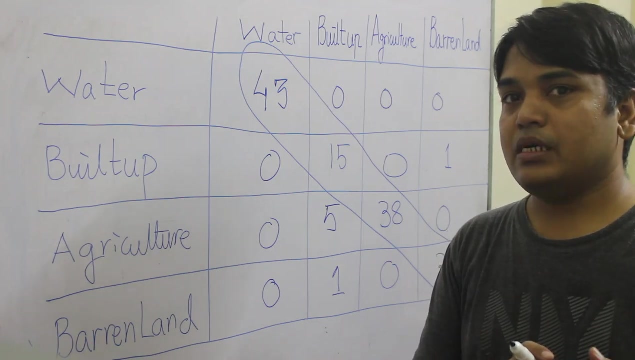 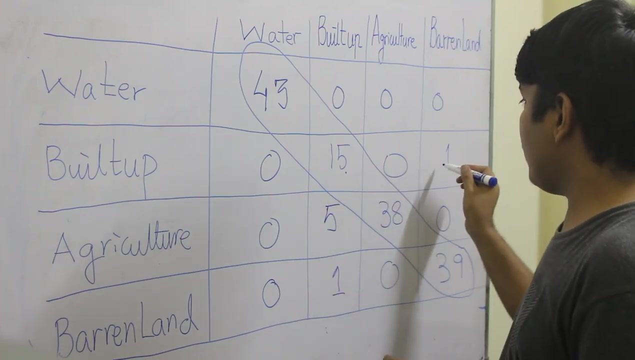 Like supervised or unsupervised classification, And then in the row you will see that we classified basically 16 samples Out of 16, 15 were actually a buildup, But 1 was very late. So what we did? we included 1 pixel. 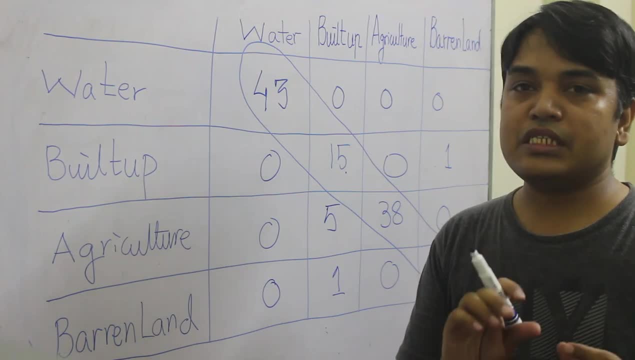 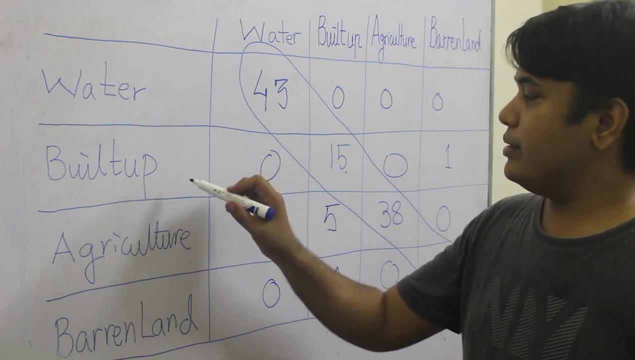 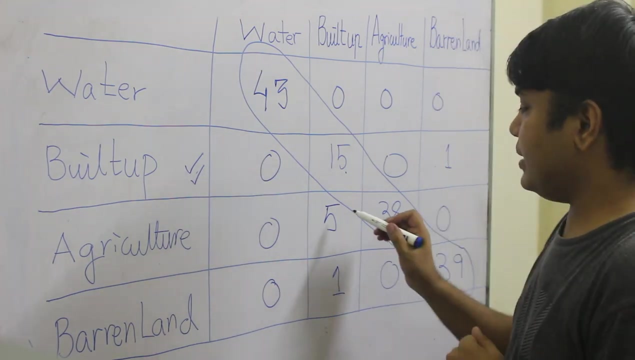 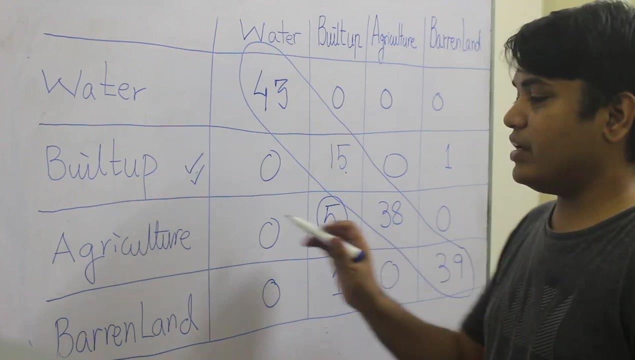 In that classification. So this is basically called commission error. So what we have done is we have included 1 pixel into the buildup area, But what happened is like we missed this 5 pixels Because we wrongfully put 5 into agriculture. 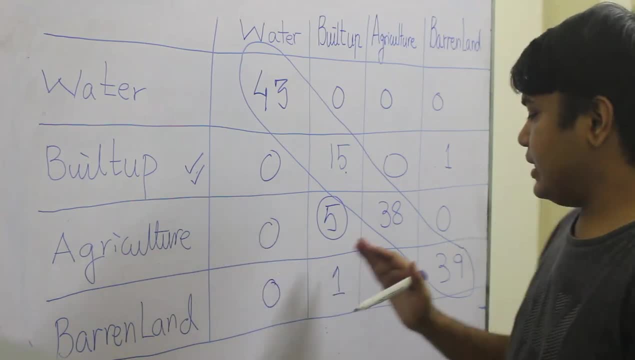 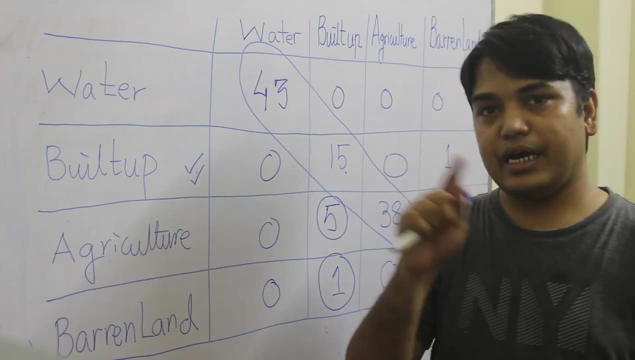 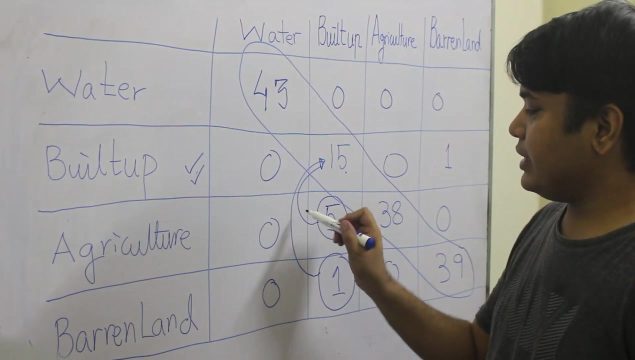 We put 5 pixels of buildup into the agriculture And 1 pixel of buildup into the barren land, So these pixels have to be a buildup class. These both have to be a buildup class, But they are actually in agriculture or barren land. 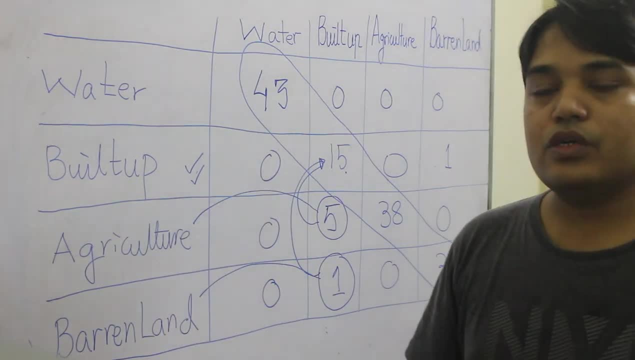 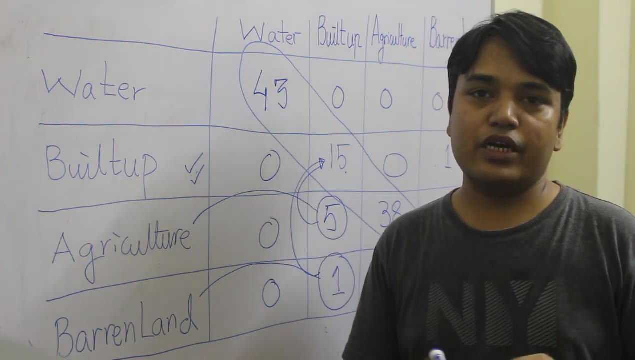 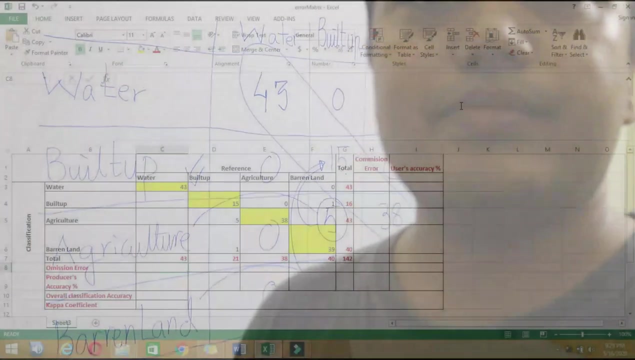 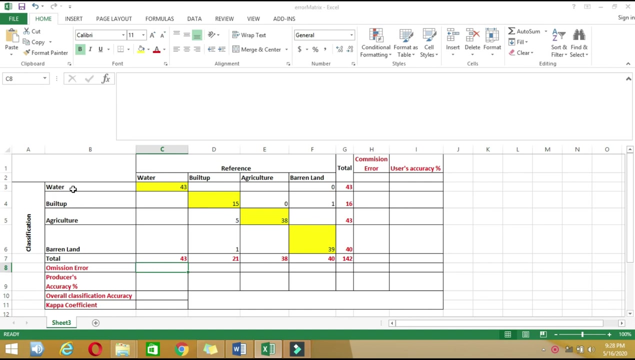 So this error is called commission error. So now we will go to our computer screen, We will put all this information into an excel sheet And calculate all other statistics. Let's see. Let's go to the computer screen. So now what we have done is basically converted what we had onto the board into an excel sheet. 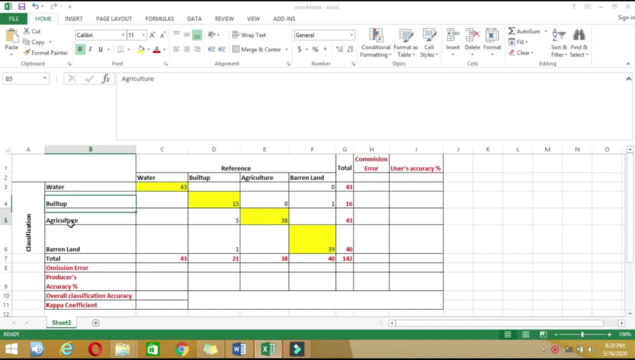 So you have classes which are water buildup agriculture, barren land, On the reference also water buildup agriculture and barren land. So in water there are total of 43 classes And also on the ground, or the reference sites, there are 43.. 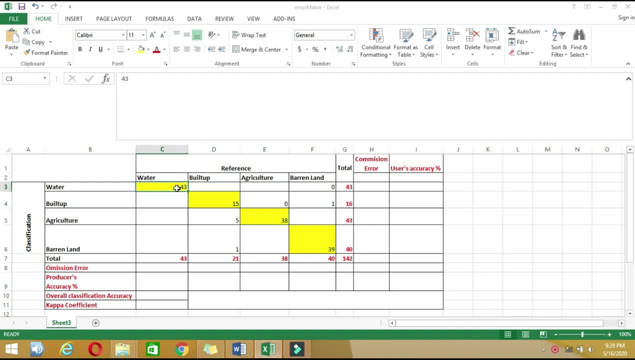 So it means they are perfectly classified by our classification scheme. And then if we see buildup, Total, 16 are classified as buildup. But if we see onto the ground, 15 are buildup and 1 is a barren land. And then in agriculture, 43 are classified as agriculture. 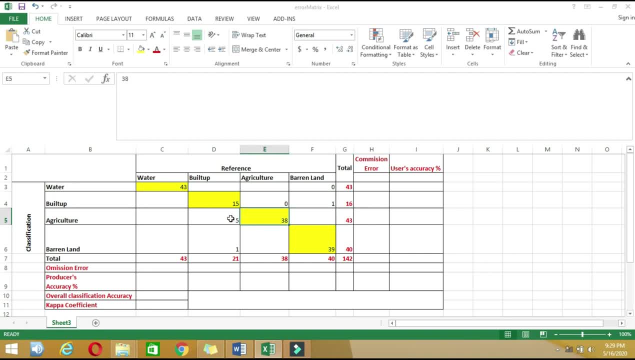 And if we see onto the ground, 38 are agriculture, 5 are buildup And then, for barren land, 40 are classified And actually on the ground, 39 are barren and 1 is basically a buildup class. So now what we will do is, first of all, we will calculate commission error. 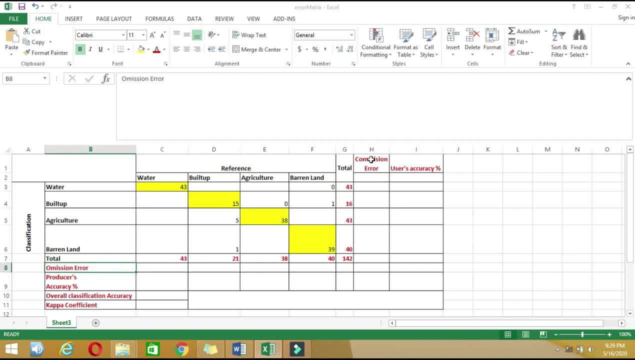 And then we will calculate commission error, Because when we have calculated both these errors, Then we can calculate producer accuracy and user accuracy, We can do overall classification accuracy And then finally we can calculate kappa coefficient. So let's first see what is omission error. 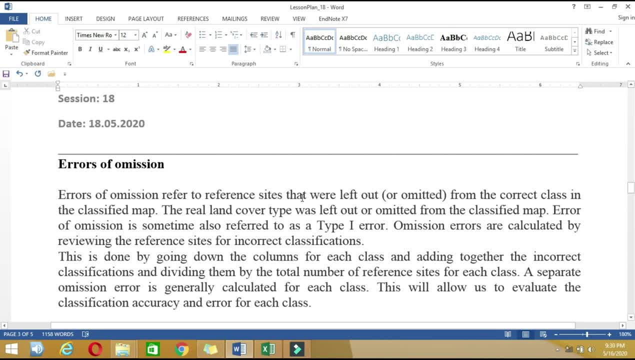 Errors of omission refer to reference sites that were left out from the correct class in the classified image. As I told earlier That these are those sites which actually has to be classified, Have to be classified as certain class but they are not. We will see in the excel sheet. 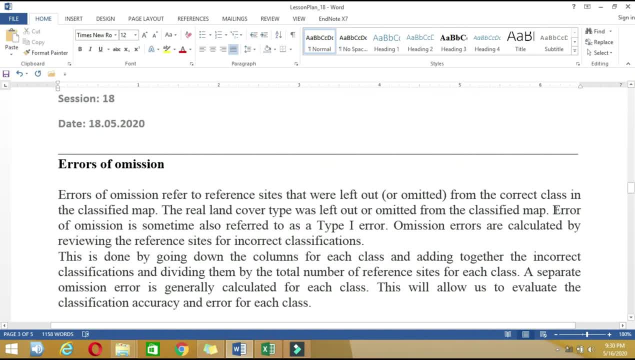 So the real land cover type was left out or omitted from the classified image. Error of omission is also referred as a type 1 error. Omission errors are calculated by reviewing the reference sites for incorrect classification. So this is the key word For reference sites for incorrect classification. 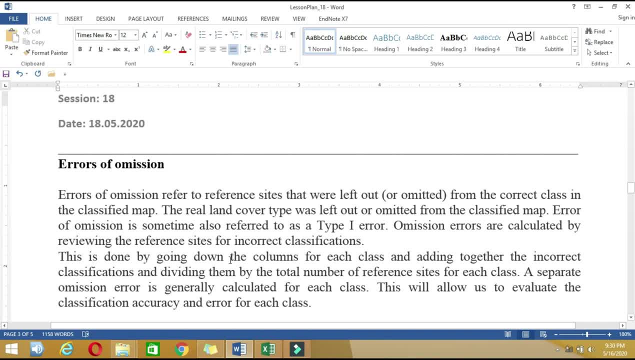 And how we have to do it. Basically, this is done by going down the column for each class, Adding together the incorrect classification And dividing them by total number of reference sites for each class. A separate omission error is generally calculated for each class. 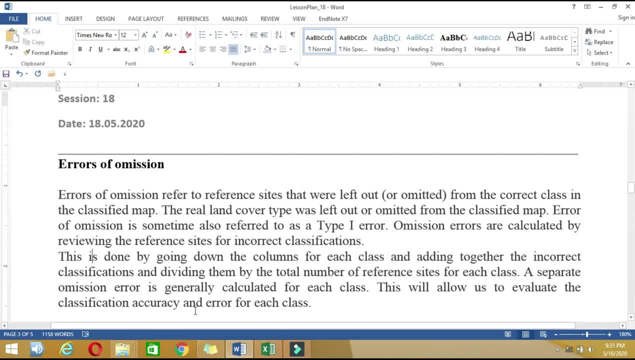 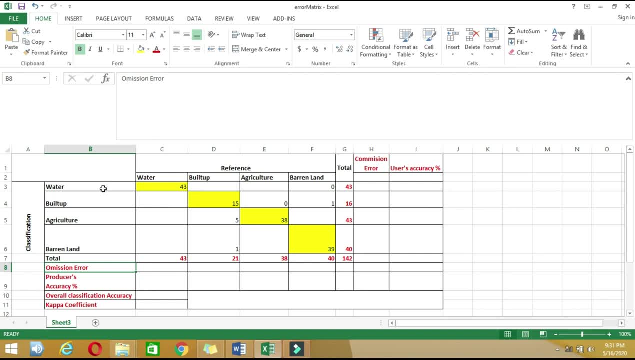 This will allow us to evaluate the classification accuracy and error of each class. So let's see it on an excel sheet. So in our water case, class In water, our classified and reference images are same, So there is not any error exists. It's perfect classification. 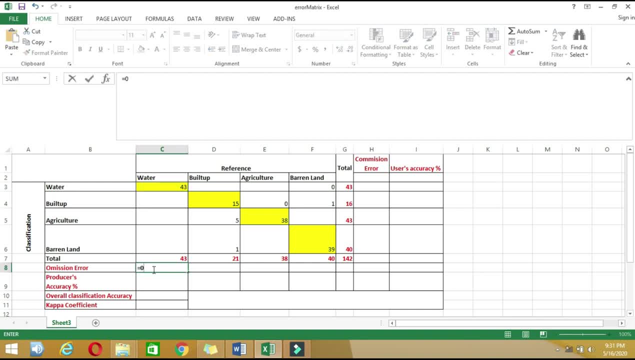 So what we have to do is basically add, So it's 0. Then we have to divide it by the total of the reference class, So it's 0. Then in this case, in build up case, we have 5 plus 1.. 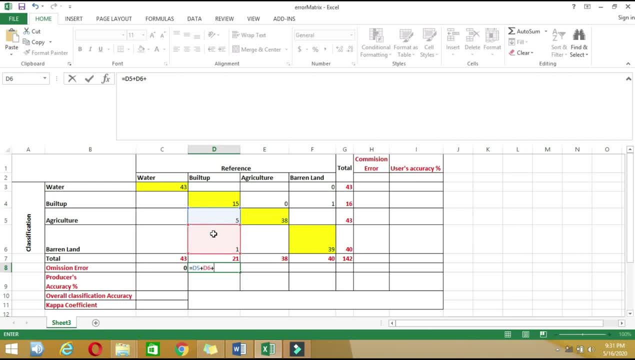 These are basically omitted from the class, So we have to divide it by the total number of reference sites. So 6 were basically not included into the class, But they are actually for build up. So what omission error to calculate is? We have to sum it both and divide it by the total number of reference sites. 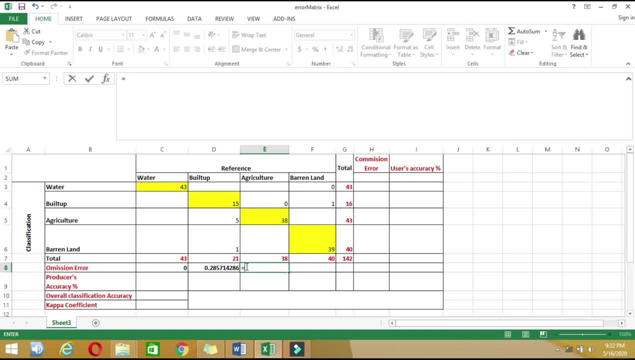 And then again we will do it for agriculture. In agriculture case it is 0.. So we will put: 0 divided by 38 is basically 0. In our barren land case it's 1.. Then plus 0, plus 0 divided by 39 or 40.. 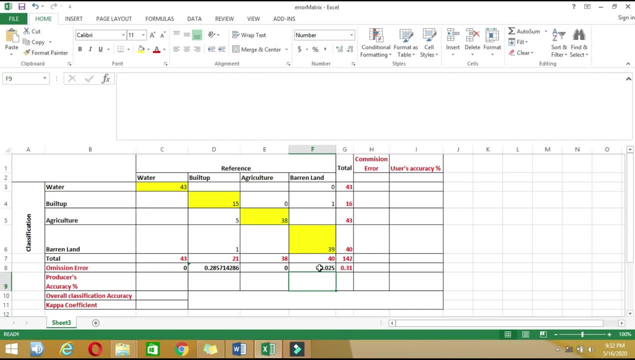 Divide by total number of reference sites, Then this is our error. So what we will do is basically: So this is automatic, We will cancel it. So you can convert it into a format of percentage, So you will get how much percentage of error you are getting. 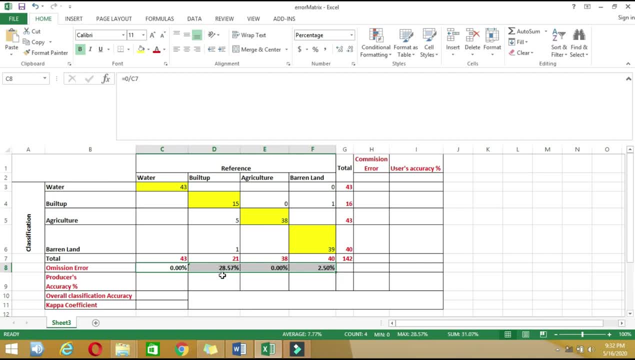 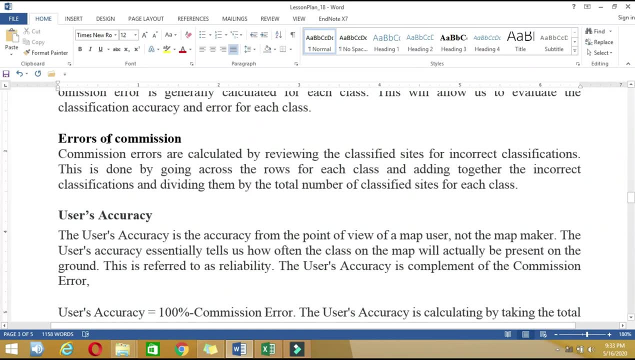 So maximum error we are getting is in the build up classifications. And now let's see what is commission error? Error of commissions, Commission error are calculated by reviewing the classified sites for incorrect classification. This is done by going across the rows for each class. 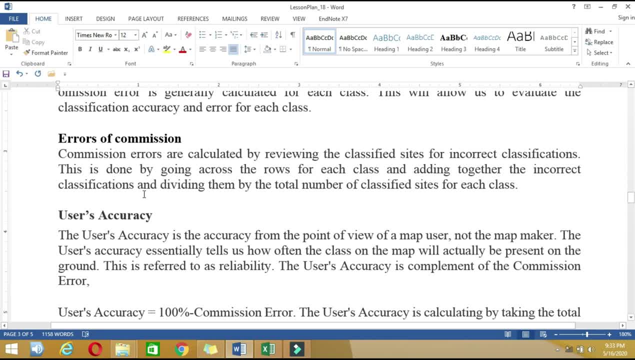 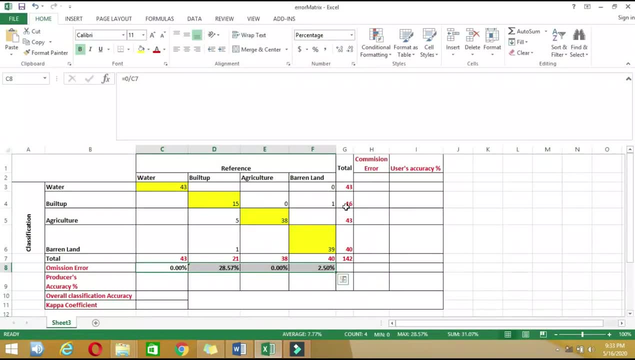 And adding together the correct- incorrect classification And dividing them by the total number of classified sites for each class. So how we will do it basically is: We will go here. So in our case, here is all 0. So we will put 0 divided by the total. 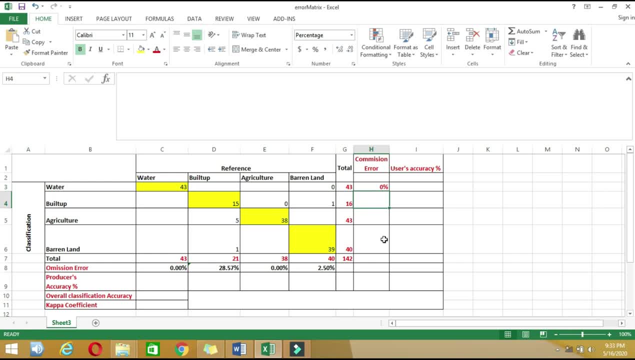 It will give us. So I have already formatted it into a percentage, So a 0 percent. Then now, where in land? So we have one incorrect classified Divided by the total, Which is 16. This is 6 percent error. 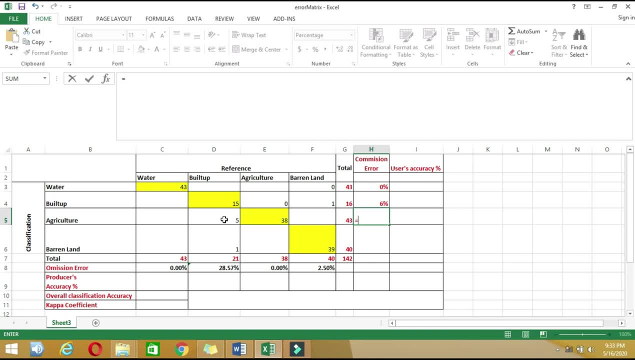 Then we will do. It's in agriculture. There are 5 which are incorrect classification. Divided by the total number of classification regions, It will be 12 percent. Then we have Barren land, Which is One is wrong classified. 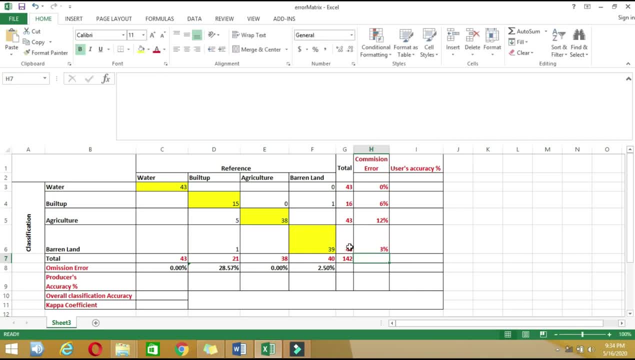 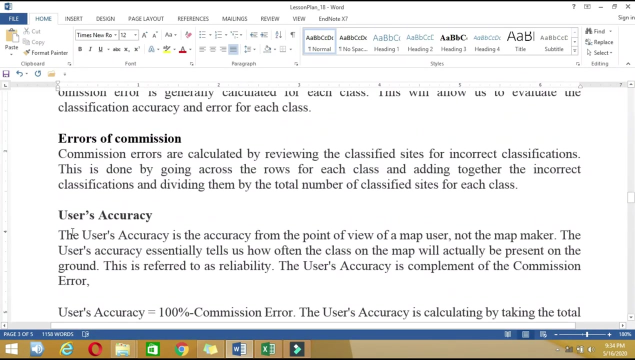 Divided by the total And it will give us 3 percent error. So you can see: here You have In commission error And here you have a commission error. Now let's see About the producer accuracy and user accuracy. So first of all, what is user accuracy? 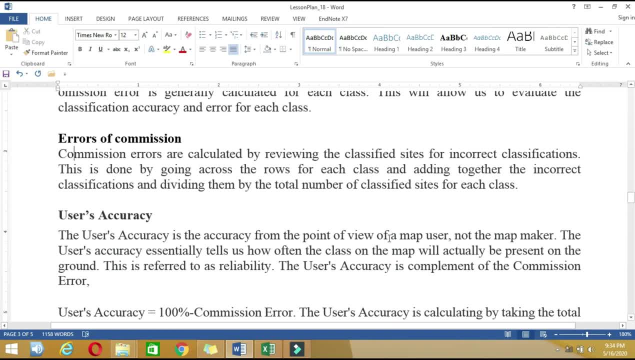 The user accuracy is the accuracy from the point of view of a map user, Not the map maker. The user accuracy essentially tell us How often the class on the map will actually be present On the ground, So This is also referred to as reliability. 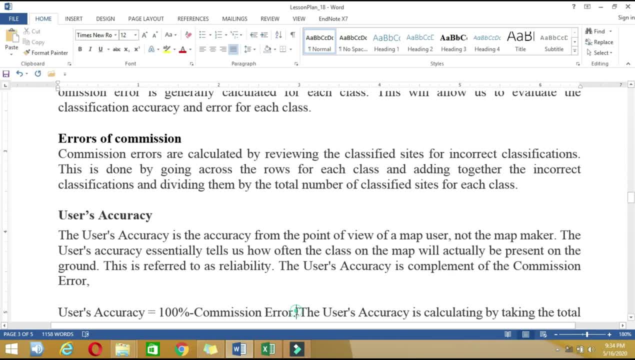 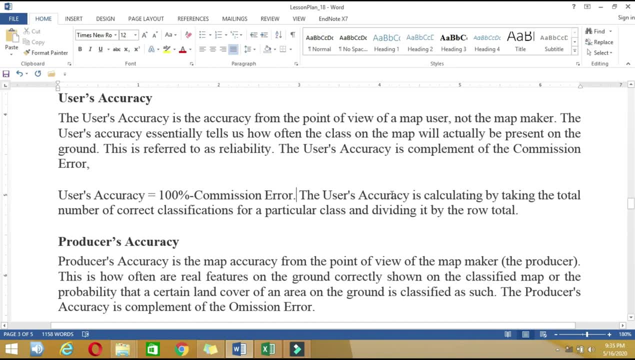 The user accuracy is complement of the commission error. So how you can calculate is basically 100 percent Minus the commission error Or the user Calculated. can be calculated by the By taking the total number of Correct classification For a particular class. 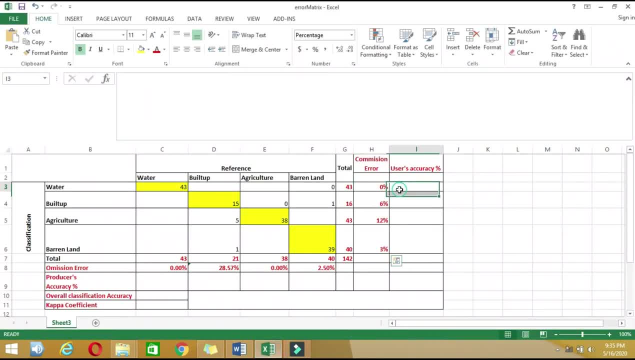 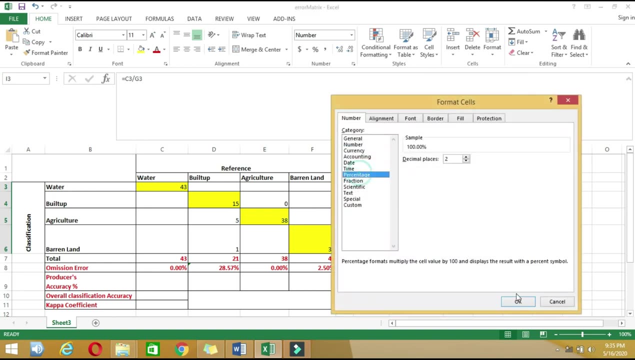 Divided by the row total. So in our case- You can see it here- Is 43.. Divided by 43. And it's 100 percent. So I can also format it into a percentage. So format Into a percentage. 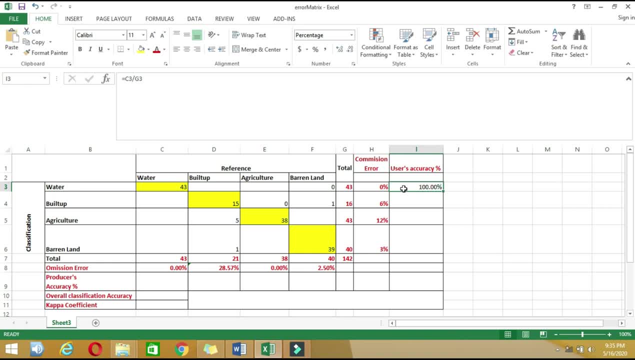 So it's 100 percent. You can also calculate The user accuracy by 100 percent Minus this. So Now This has to come: 94 percent Calculate by the Above formula 15.. Divided by: 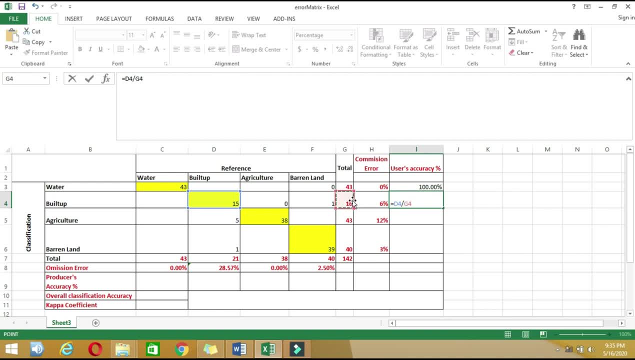 16. So it's approximately 94 percent. Then again you can do it: 38. Divided by 43. Is 88.37 percent. Then you can calculate 39. Divided by 40.. 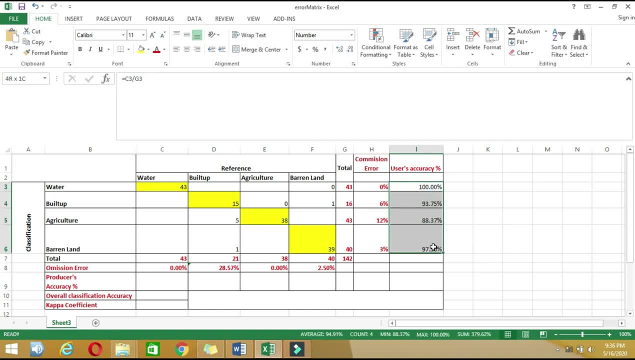 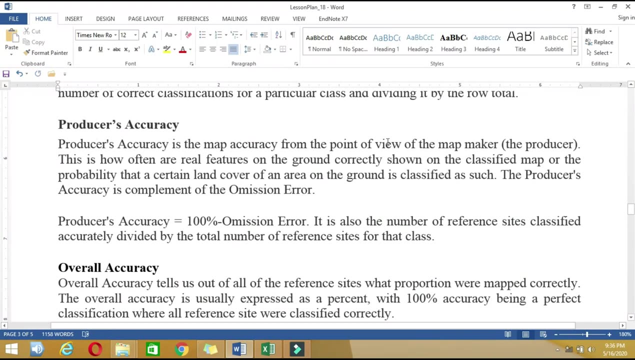 It will give you. So this is your user accuracy For your classification scheme. Now let's see What is producer accuracy: Producer accuracy From the point of view Of the map maker, The producer, This is how often Are real features. 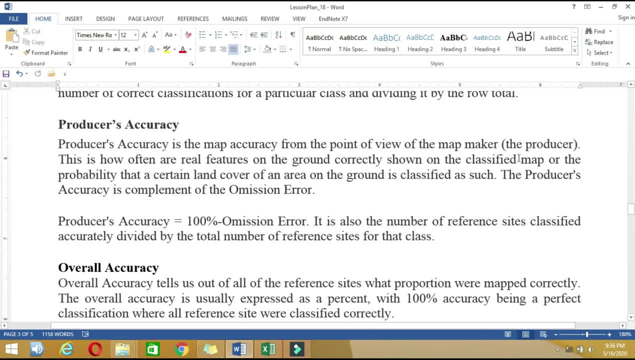 On the ground Correctly shown On the classified map, Or the probability There is a certain Land cover Of an area On the ground Is classified As such. Producer accuracy Is complement Of the omission error, So producer accuracy. 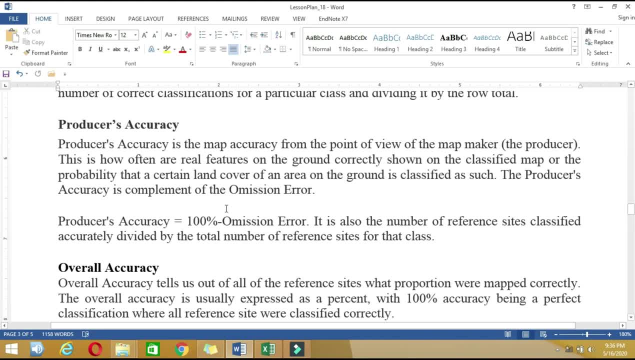 Can be calculated By 100 percent Minus The percentage Of the omission error, Or We can calculate It by The percentage The number Of reference Sites Classified Accurately Divided By. 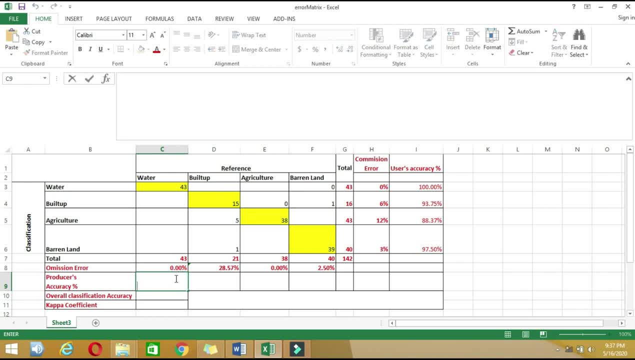 The total Number Of reference Sites. So We will. So These are The correct Classification Divided By The total Number Of reference Sites. We will Also Convert It Into: 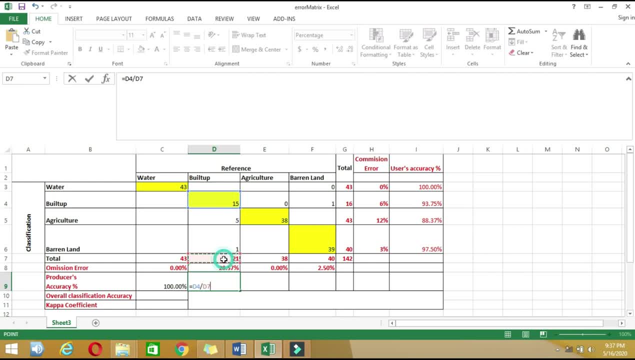 A, Divided By The reference Classes, It Is 21.. Again Then You Have Can Calculate 38. Divided By The 38. So It's 100 percent. 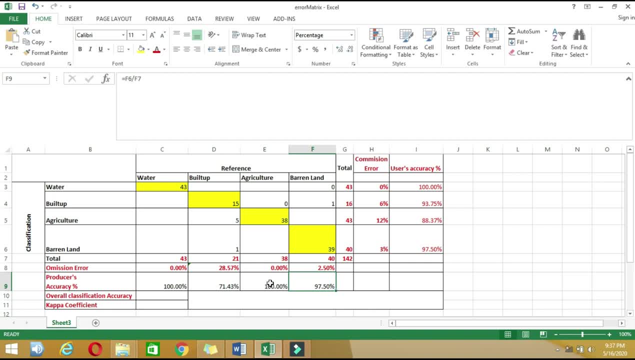 Then You Have 39. Divided By The 40. You Have By The total Sites And Or By 100.. Percent Minus. So This Is Really. 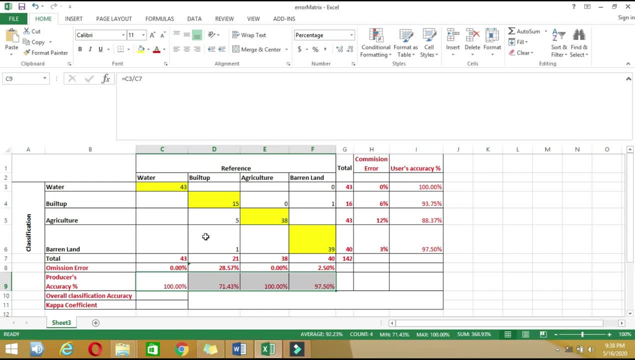 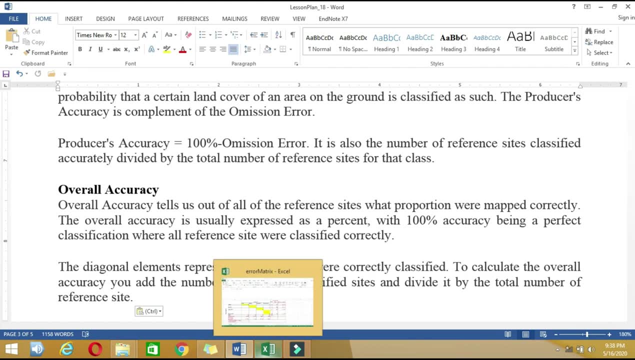 Like Good Tool To See How Much Error You Are Having Classification. And Then There Is. So It's Basically The Crack Side Percentage, How We 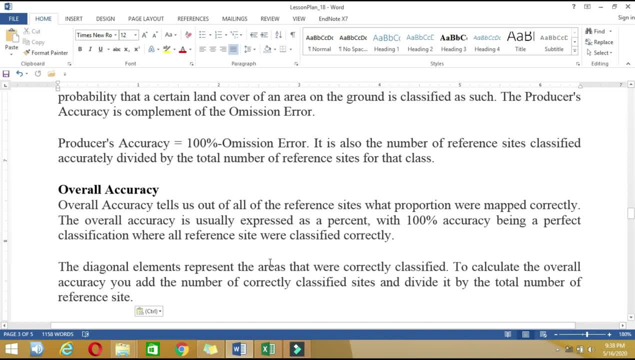 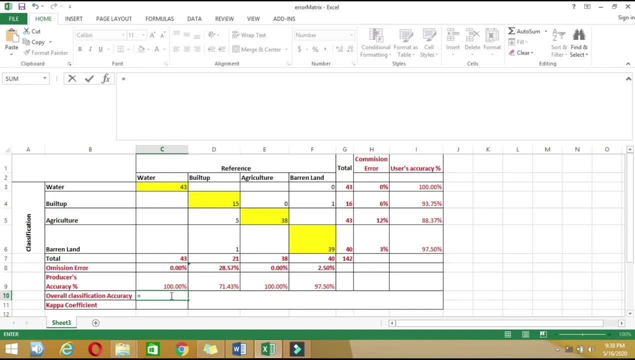 Will Calculate It. So We Will Add All The Diagonal Diagonals, So, And Then We Will Divide It By The Plus This, Plus This. 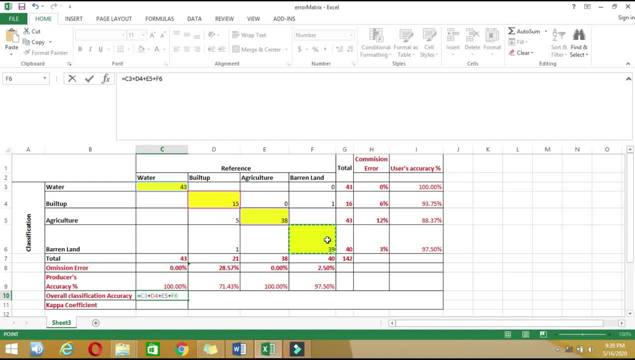 One All Diagonals, Then We Can Put It Into The Bracket. Then We Divide It By The Total Number Of References. So In Our Case, 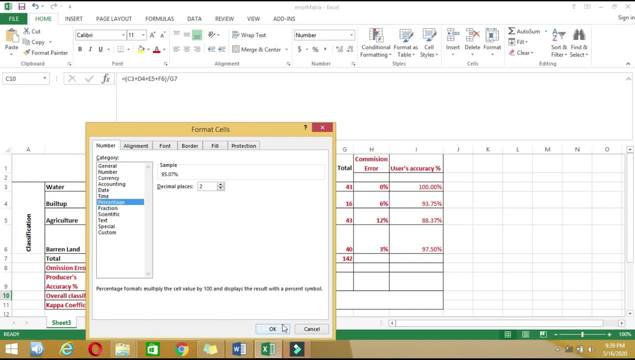 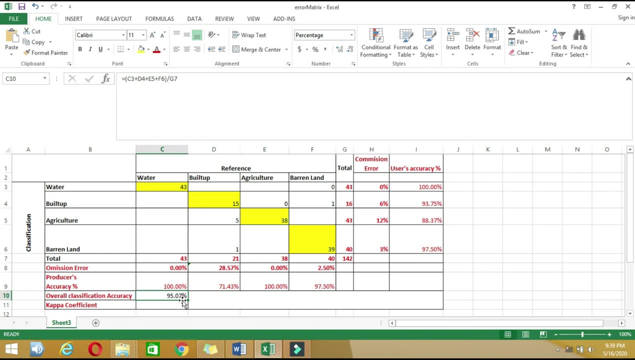 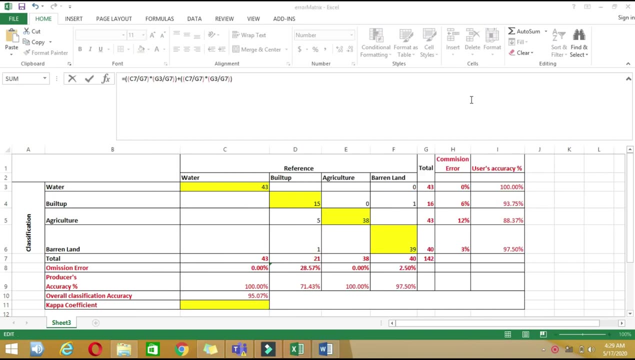 We Have A Very Good Thank You For. So It Is 95% Of 95.. 107% Of Classification Accuracy. So Now What We Will Do. 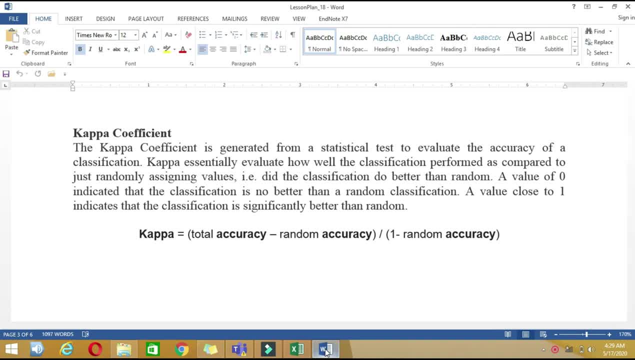 Is Calculate Copper Coefficient And Copper Essentially Evaluate How Well The Classification Perform As Compared To Just Randomly Assigning The Values. Is That Did? 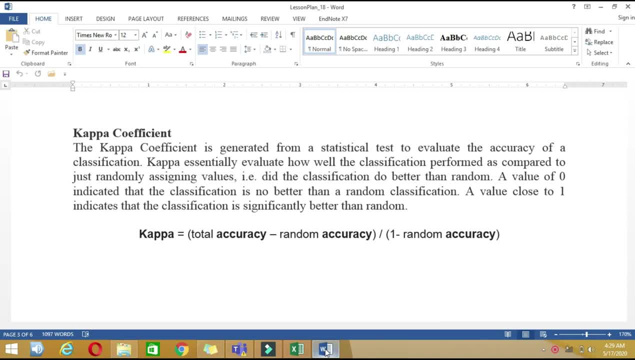 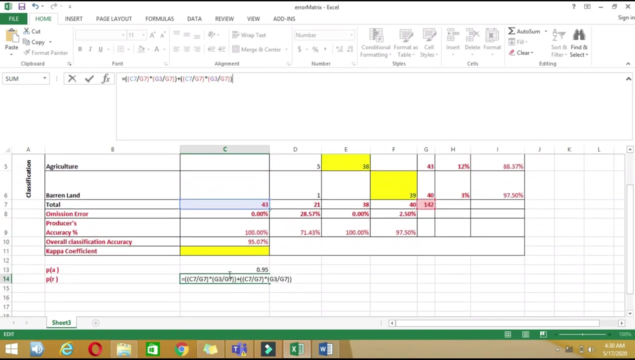 The Classification Do Better Than The Random. A Value Of Accuracy. You Subtract Random Accuracy By From Total Accuracy And Divided By One Minus Random. 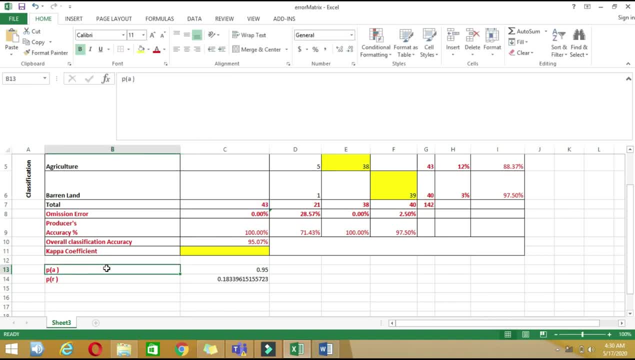 Accuracy And How To Do It On Excel Sheet. Let's Consider That You Have Your. You Need To Calculate Your Random Accuracy, So I Will. 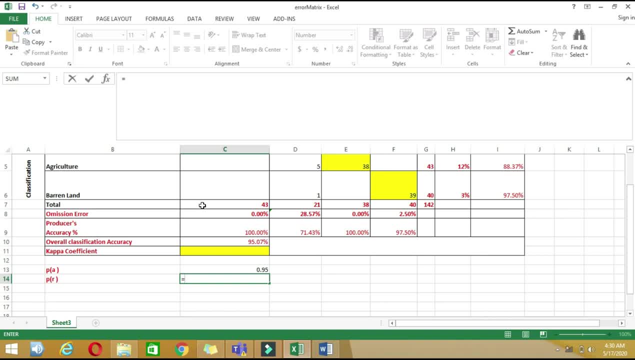 Do It Basically Is So We Have To Take Our Total Of Column Divided By Total Reference Sites, And What I Have To Do Is 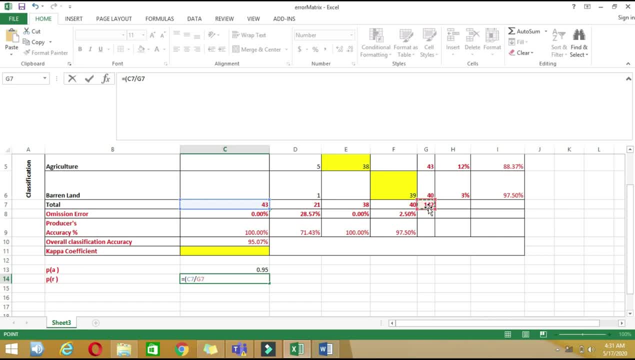 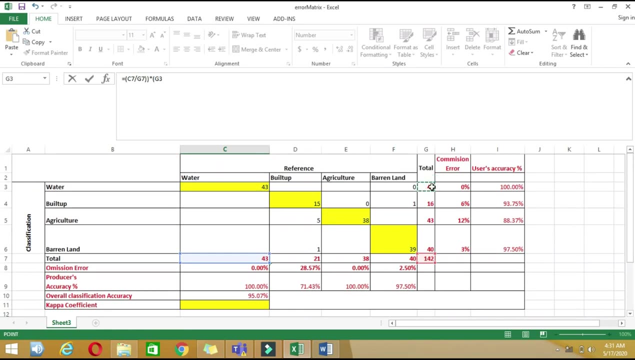 Basically Take This Divided By The One, Forty Two, Then Multiply It. Multiply It By The Row. Total Divided By The Total Divided By. 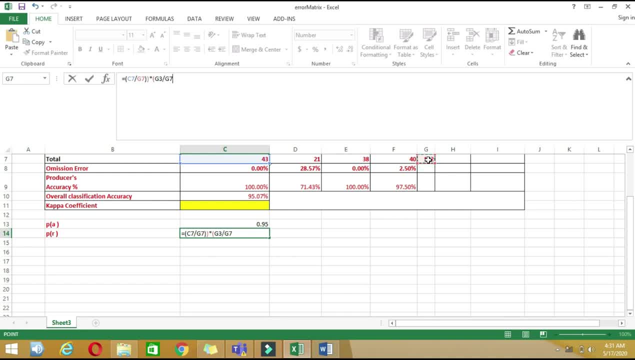 One, Forty Two Again, Then We Will Do Same For All Other Classes. So This Was For Water. Now We Will Add And Do It For. 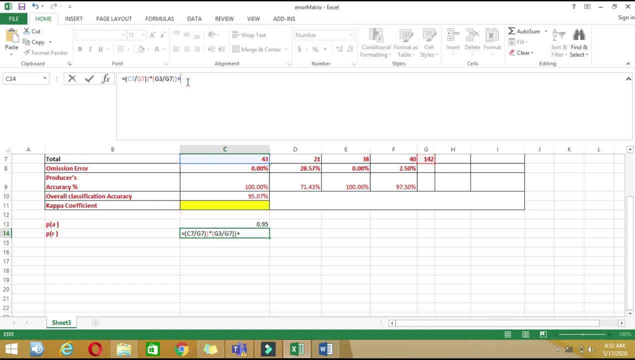 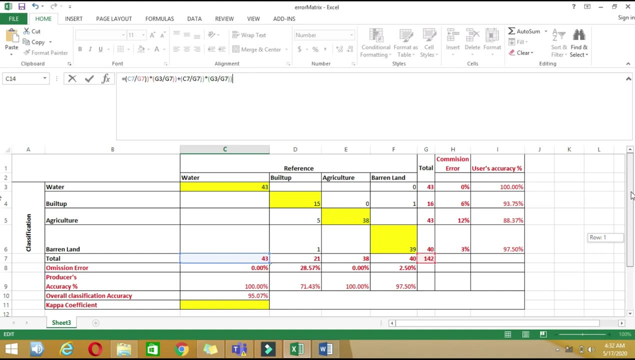 Other Ones Now I Have. So My Build Up Is In D Seven And G Four, So Converted Here To D Seven And G Four. So 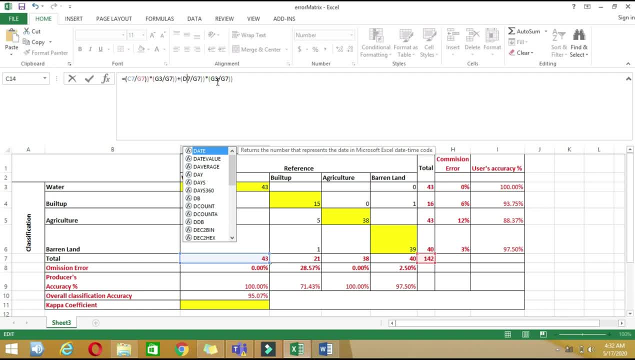 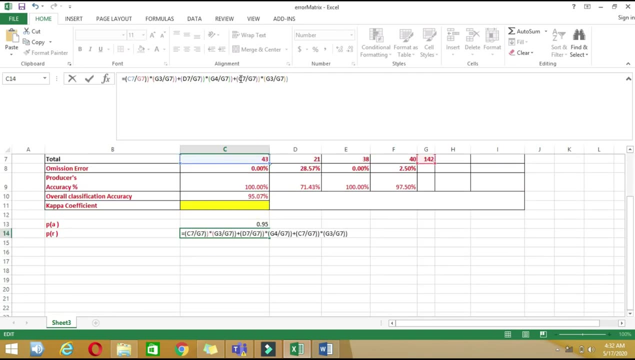 Converted Here To D Seven And G Four. Now The Same For Will Do Same For Agriculture. So Our Agriculture Is In E, Seven And G. 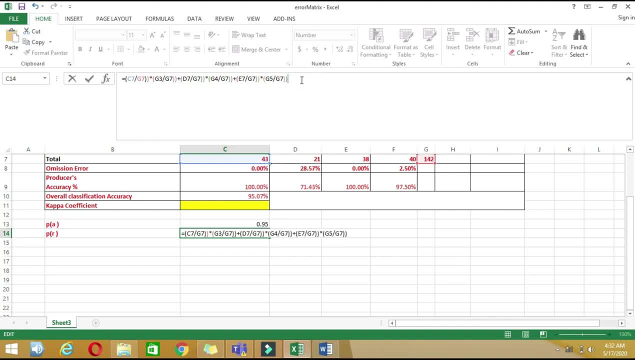 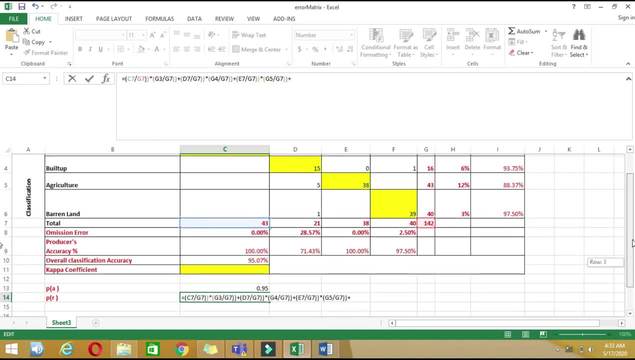 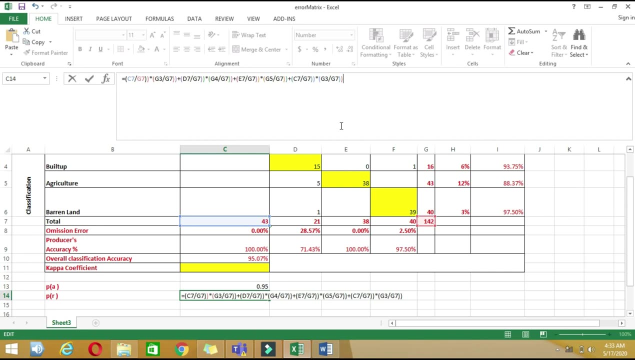 Five, Then Will Do Same. Your Final Class, Which Is Basically By Land, And It Is In Its Total Is In F Seven And G Six. 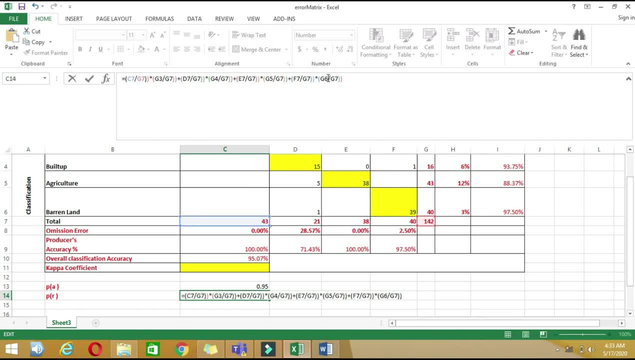 So We Press Enter, So Press Enter. So Okay, There Are Some Brackets Missing. Let's See, Here Is One Of Our Bracket Missing. It Will. 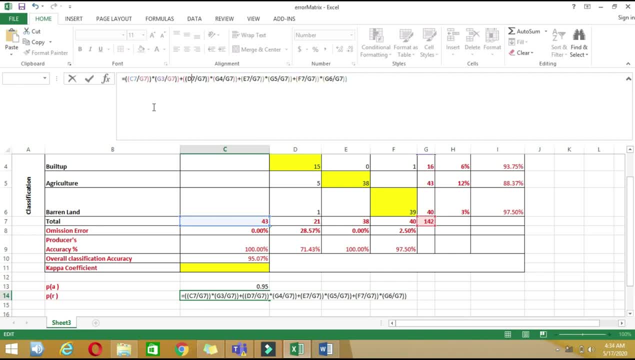 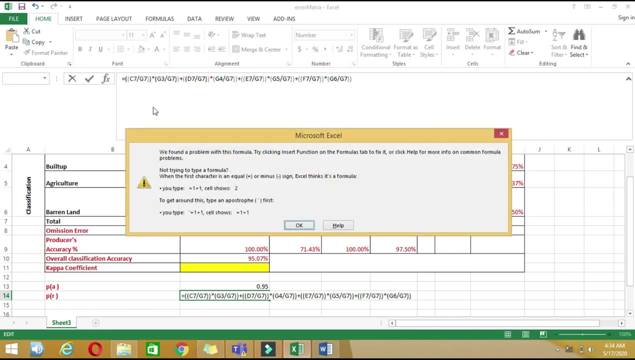 Be Missing. In All Over Completed. Some Formatting Mistake. Brackets Are Missing. Now- Now I Hope It Will Work Again. Some Brackets Are Missing. 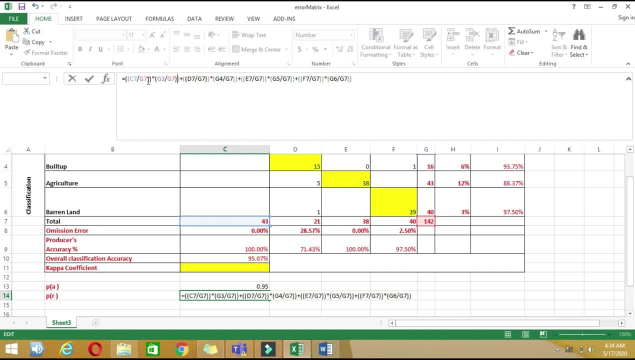 Let's See Where Are We Missed. So This Looks Okay. Then Close This Whole Bracket That Added. So An Extra Bracket Here, Extra Bracket Here. 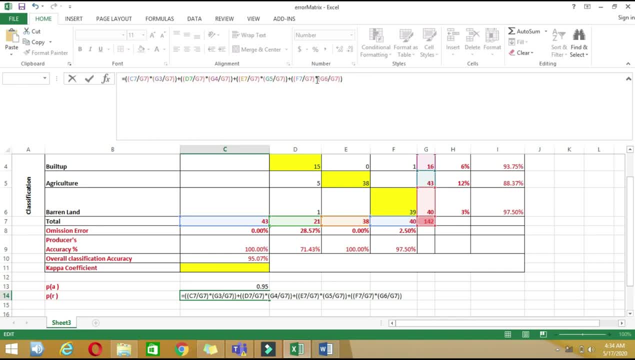 An Extra Bracket Here, Press Enter. Now We Have Calculated This Random Accuracy. Just To Check, What You Have To Do Is Basically Multiply Your. 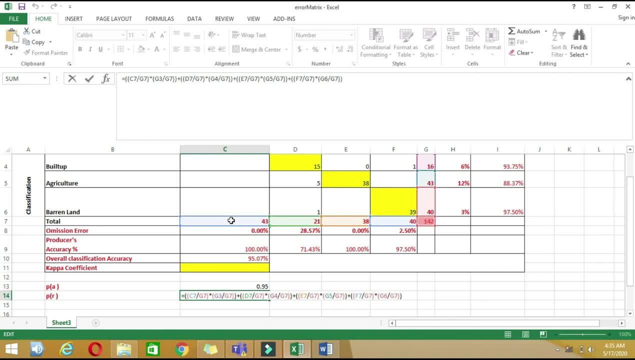 Column Totals By Divided By The Total Reference Side, Then Column Total, Then Row Total Divided By, Then Add All To The P A. 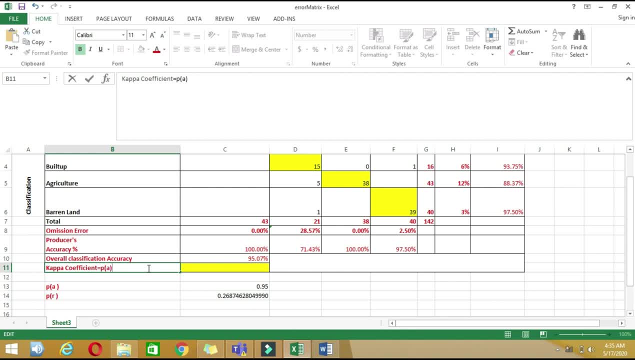 Minus P? R Divided By One Minus P. R Divided By One Minus P. R. P R Divided By One Minus P. 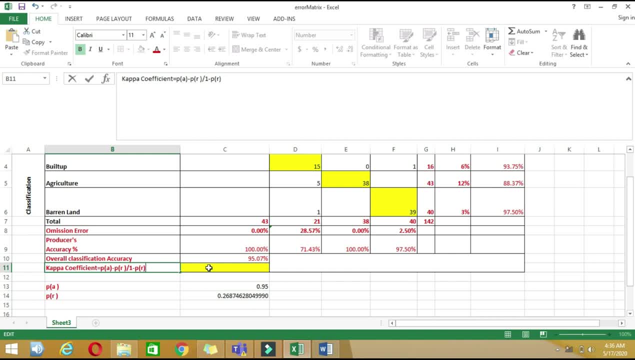 R, The. so we will calculate it here. so what I want to do is this minus this. put it into the brackets, then we will divide 1 minus PR, close into the brackets and press enter. so this is our copper coefficient, which is 0.93, which is actually good one. we can see it from. 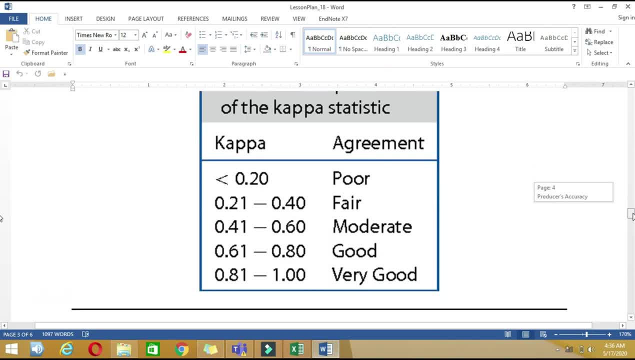 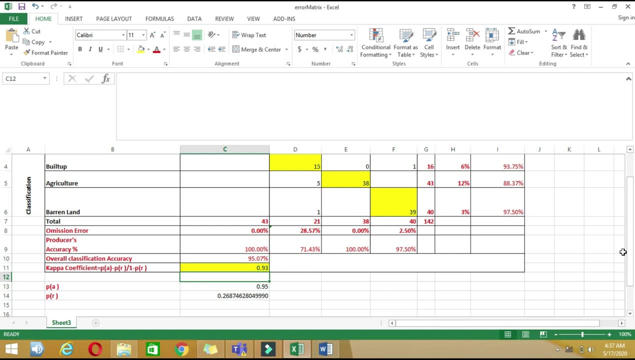 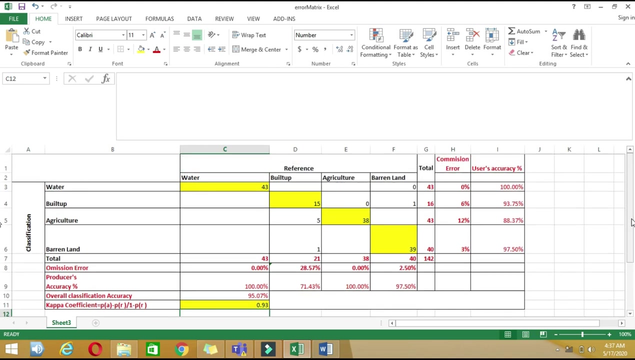 this table. so if your copper coefficient is near to zero, it's poor, and when it's near to one, it's very good. so in our case it's really good copper coefficient. and now we have calculated all of the statistics and completed our error matrix. just to revise briefly, so you have. 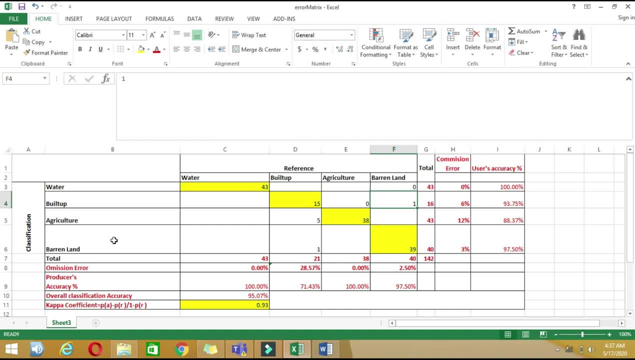 your classes, what are built up, agriculture. then in rows you show your classified, your results through your classification, and in columns you show your reference sides by ground truthing, and then you take column or a row total and a column total. then you calculate omission error and commission error. commission error is the error in which